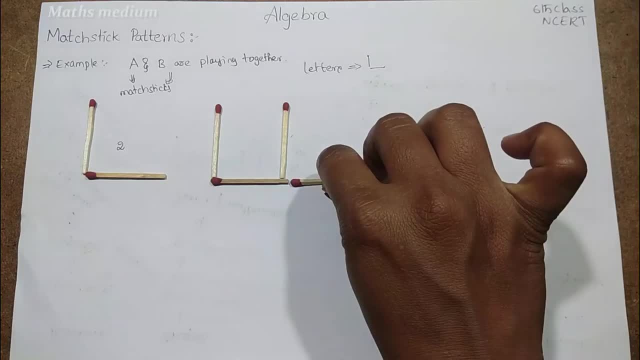 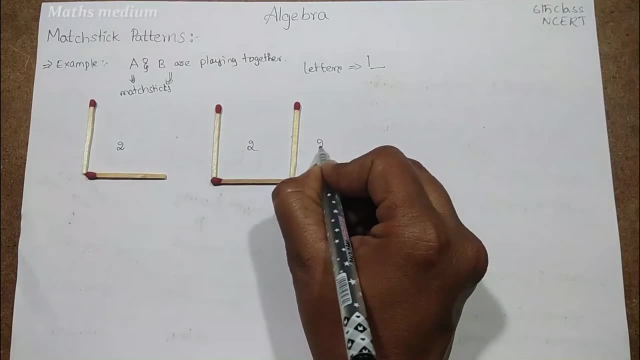 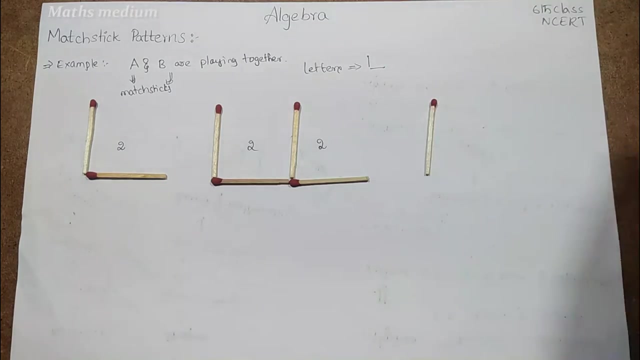 So this is one L and this is another L. See, if you observe, and here we need two and this is also two. Next, they are started forming like this. So another shape is like this: See one, two and three. 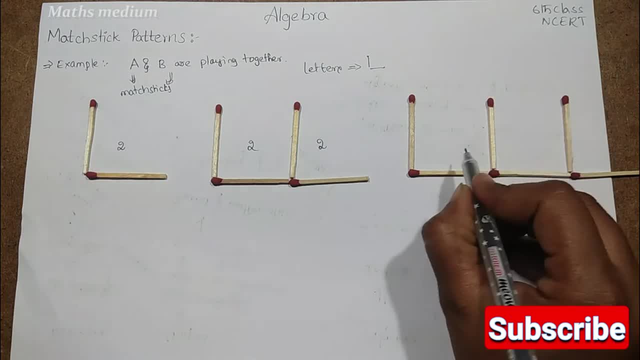 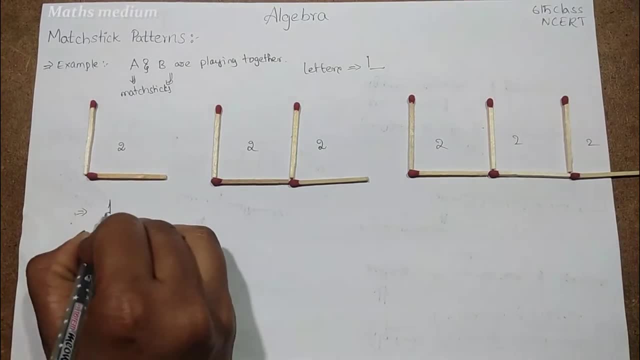 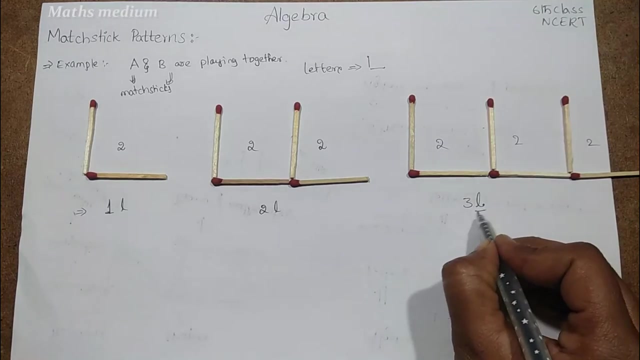 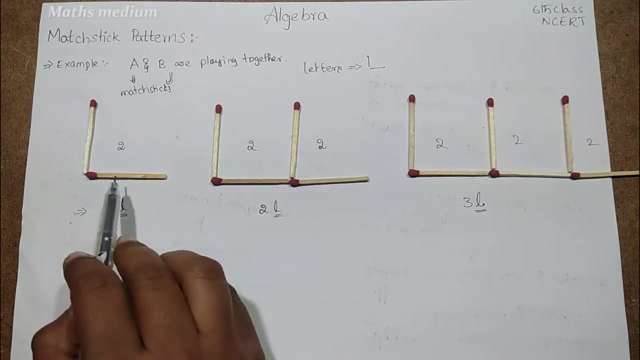 like this right. So how many Math Sticks here needed Two plus two and another. So how can we call it as this? one L, This is two L, This is three L in terms of algebra. So algebra needs small case alphabets. So that is not a fixed value. But here see one L, two L. 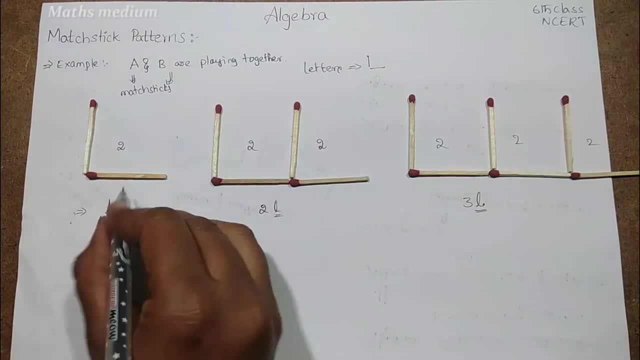 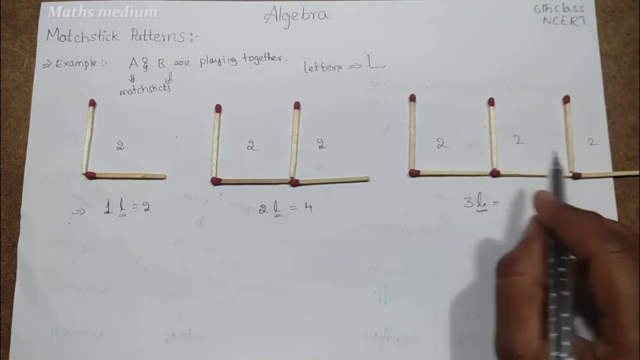 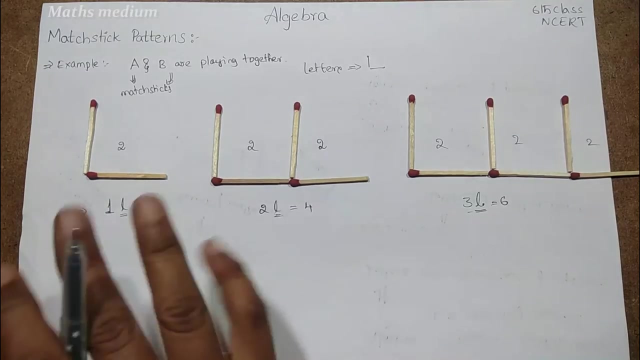 three Ls In this one L. how many Math Sticks we need Two In this two L. how many Math Sticks we need Four In this Math Stick pattern? how many Math Sticks we need six right. So two, four, six for three L and two L, one L Math Stick pattern. 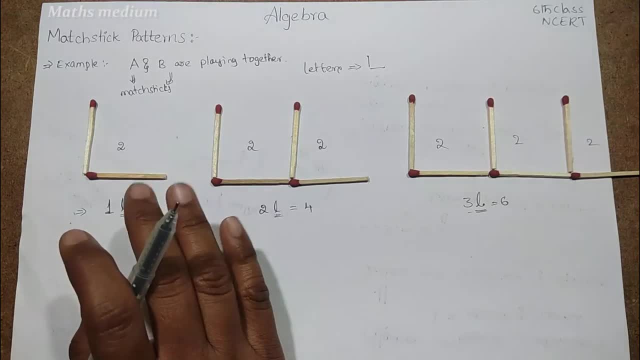 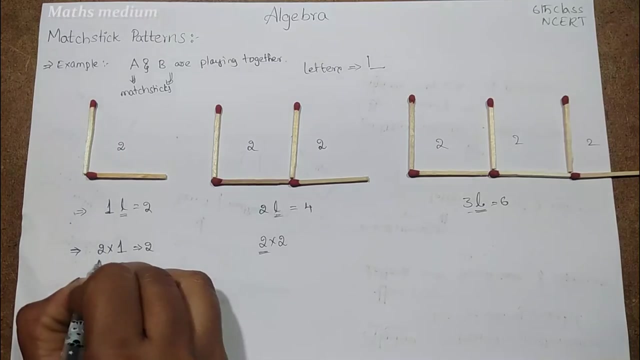 Now how we are going to transfer this into form of a expression, like by using any letter. So here, two into one L. So that is equal to two Here two into two. Here two means two Math Sticks. 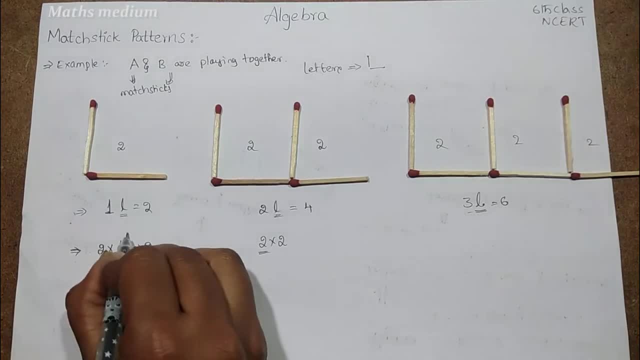 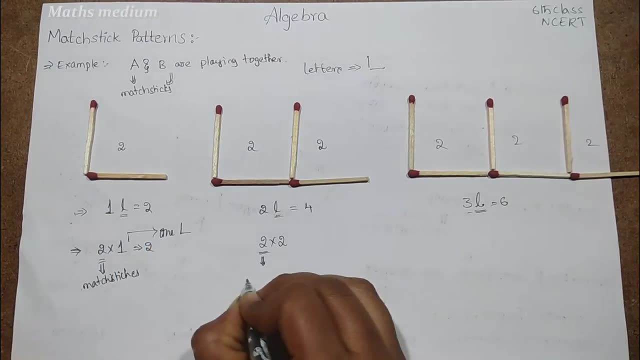 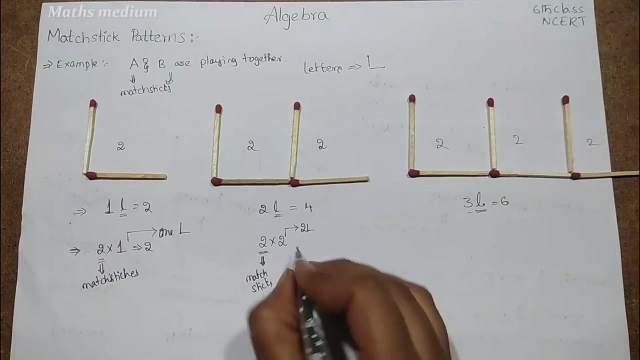 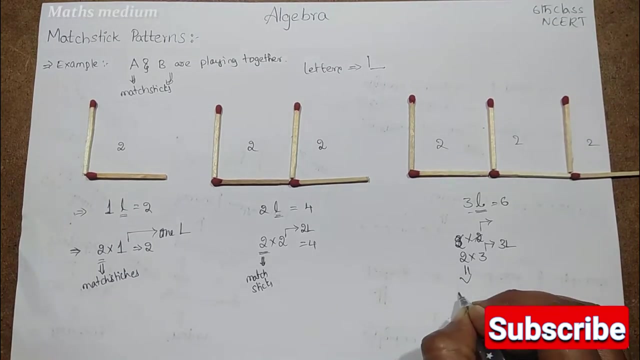 Here one meets one L. Okay, Here also two Math Sticks. Here we are forming two Ls. So that is why four L Here, two into three, Here three L, and this is two Math Sticks. 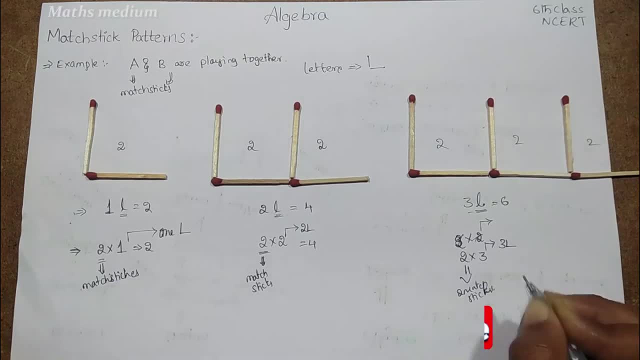 So by observing this, if we need N patterns, how many Math Sticks? we need Two Math Sticks with N patterns, So this is called two L If you want five, if we want five L pattern, then how would we? 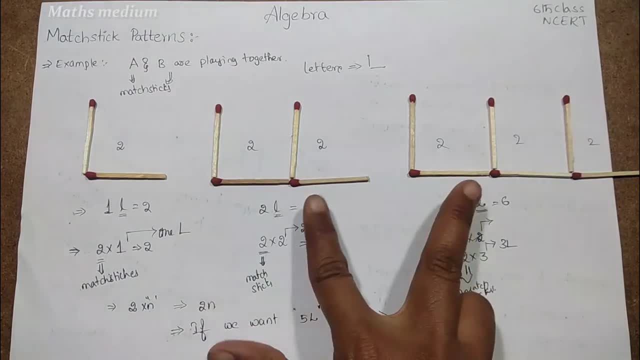 see, If you add these two, it means two Ls, So this is called two Ls, So this is called two Ls. So if we add these two, it means two Ls, So this is called two Ls, So this is called two Ls. So 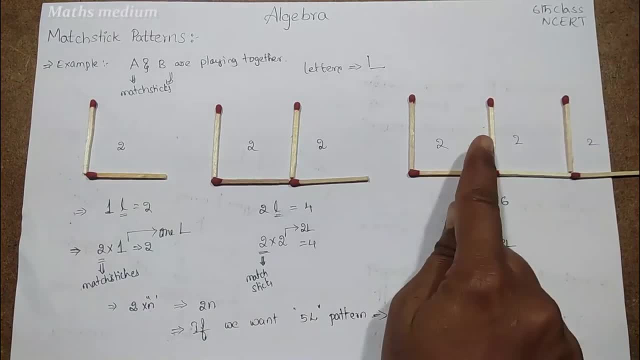 we get five right: One, two, three, four, five, six, seven, eight, nine, ten, Ten Math Sticks we need, But in practically here with this formula, that means this rule, we can call it as: 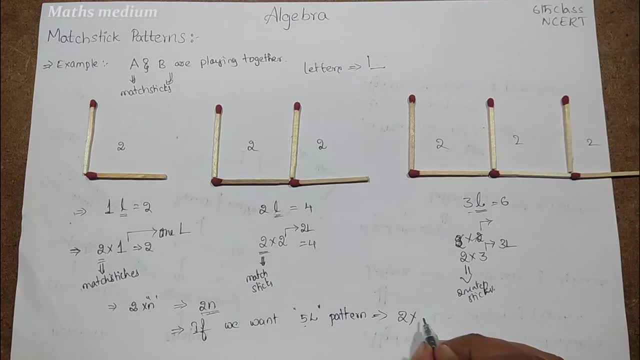 two into how many patterns? Five, It means five, This is ten, right? So similarly I want eight L patterns. so how many matchsticks do we need? so please comment in comment section. i hope you understand about this session. if you have any doubts, comment on comment section. please click like button share. my videos and subscribe my channel, thank you. 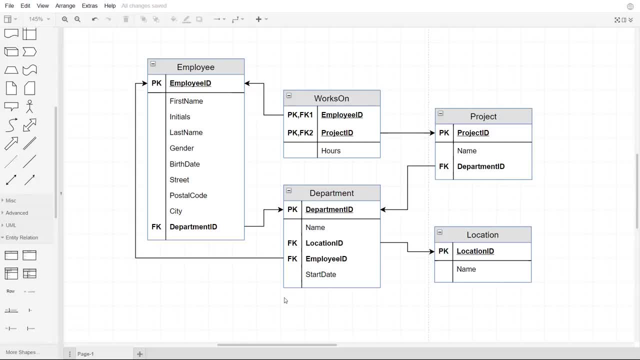 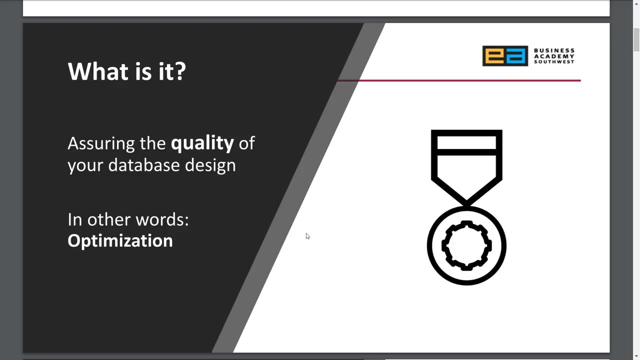 Hey everybody and welcome to this video about how you can normalize a relational data model. We have this, this RDM, here that we will use to normalize and basically normalization is about how we can optimize the database. It is about assuring the quality of your database design and an important part is 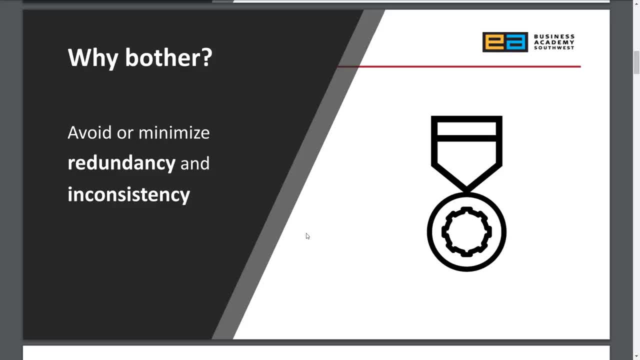 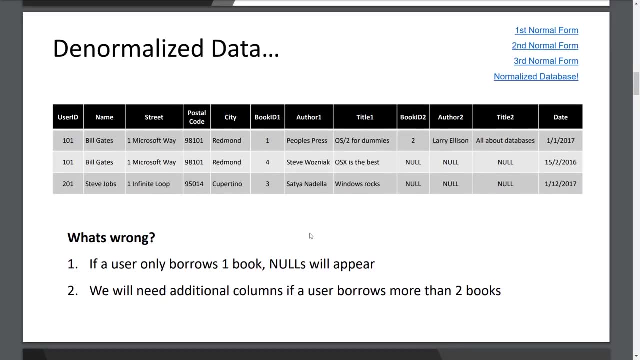 that we can avoid. we should avoid or minimize redundancy and inconsistency, so we need to avoid extra data, duplicate data, null data and, if we should take a quick look at how a denormalized data could look like, this is a good example, where we have a lot of null values and we just have one table and we have we. 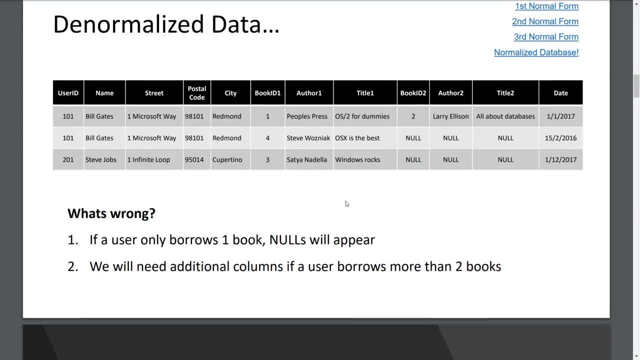 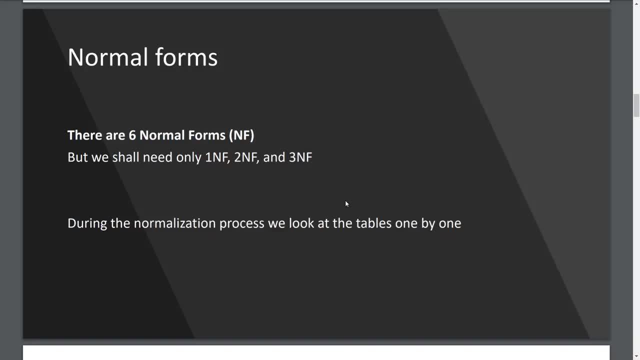 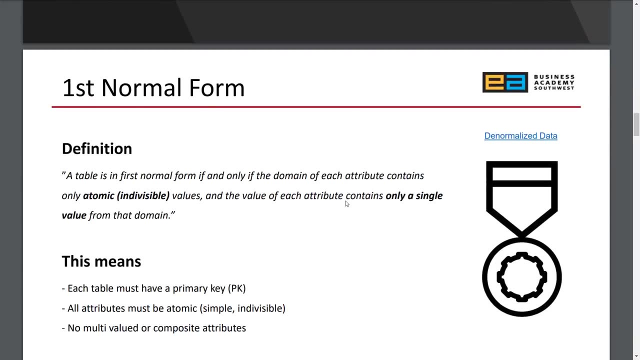 haven't split it in in any further tables to normalize something. we well, we have six normal phones, but I'm gonna normalize this to to the third normal phone and during this normalization process we look at the tables one by one. so if we we should take a look at the